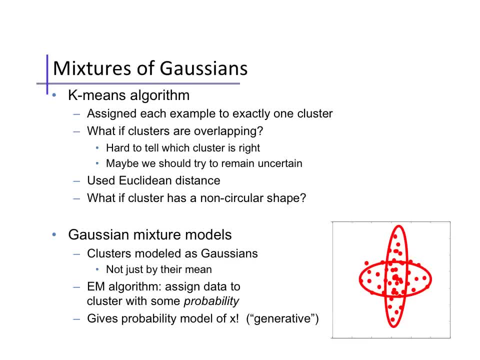 Both are centered at the same place, So it's easy mentally to see these as falling into two groups and to cluster these data in one and these data in the other. But something like k-means won't be able to discover that assignment. 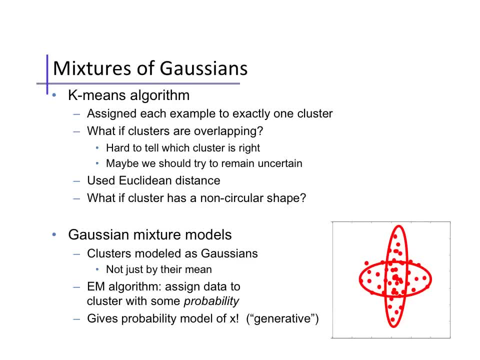 Gaussian mixture models are an extension of the k-means model, in which clusters are modeled with Gaussian distributions, So we have not only their mean, but also a covariance that describes their ellipsoidal shape. So then we can fit the model by maximizing the likelihood of the observed data. 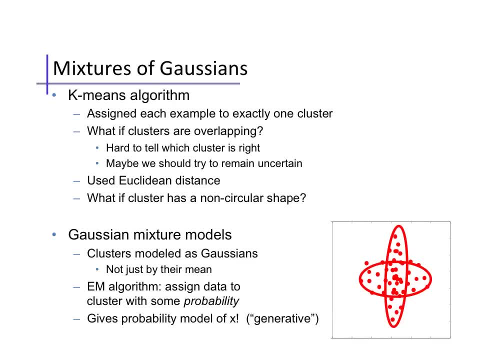 We do so with an algorithm called EM. It'll be very reminiscent of k-means, except it'll assign data to each cluster with some soft probability As a positive side effect. after clustering, we're actually creating a generative model for the data x, a probability model. 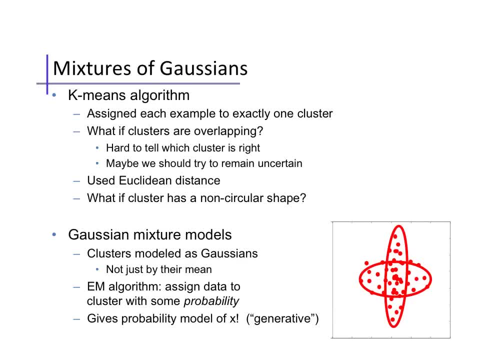 Which means we can do a lot of useful tasks Like sampling new examples that we think are like the data that we measured, Or comparing two collections of data, like the training and test set, to see if they differ, Or imputing missing data values from some of our data. 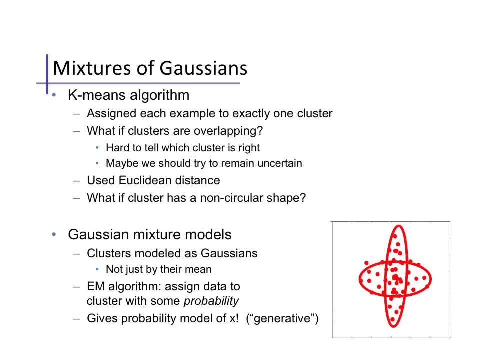 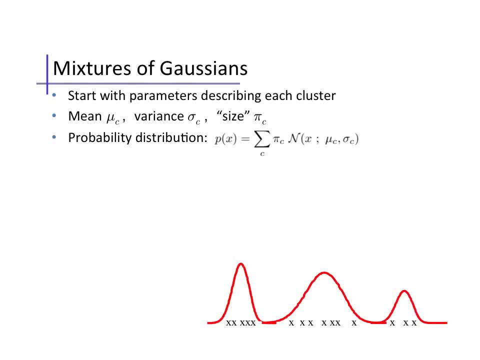 In fact, often k-means is actually viewed as a special case of a Gaussian mixture model. to derive some of these benefits, A Gaussian mixture model is a useful probability distribution model. We begin with several mixture components Indexed by c, Each of which is described by a Gaussian distribution. 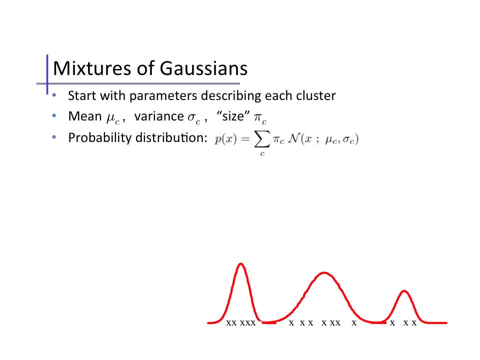 So each has a mean mu c, A variance or covariance, sigma c And a size, pi c. For example, in this figure we have three Gaussian components, Which means here, here and here. Each of these components has a different variance. 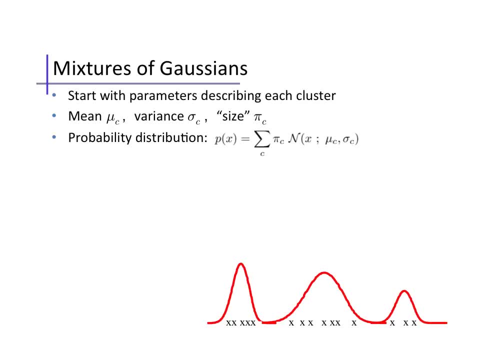 And a different height or area. So the joint probability distribution model is then defined by the weighted average of these individual components, So pi c times the Gaussian, defined by mu c and sigma c. We can interpret this joint probability distribution over x in a simple generative way. 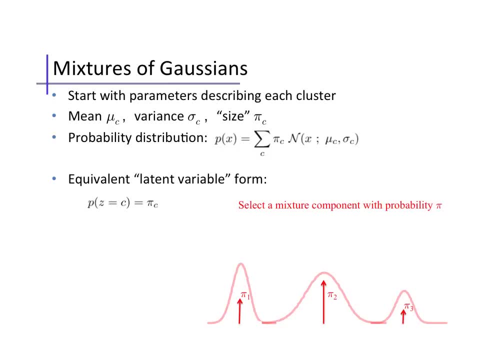 To draw a sample from x, from p, we first select one of the components With discrete probability, pi. So components with large pi are selected more often. As in k-means, we'll view this as the assignment of that sample to one of the components and denote it by z. 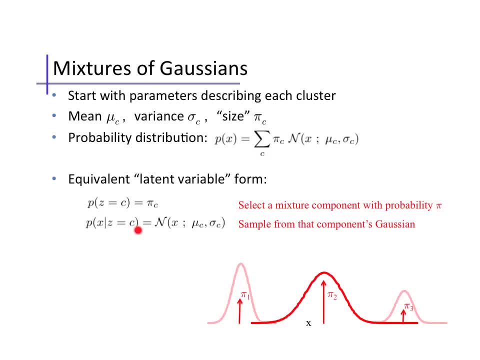 Then, given the component assignment z equals c, we can draw a value from x from the corresponding Gaussian distribution. So together these two distributions make a joint model over x and z. Discarding the value of z gives a sample from the marginal p defined above. 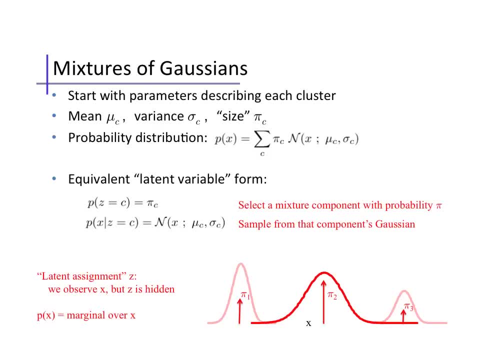 Models like this are sometimes called latent variable models. The data x are modeled jointly with an additional variable, z, that we don't get to observe. it's hidden. The presence of the unknown value of z helps explain patterns in the values of x. 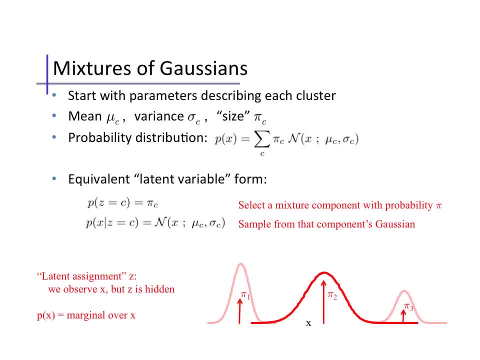 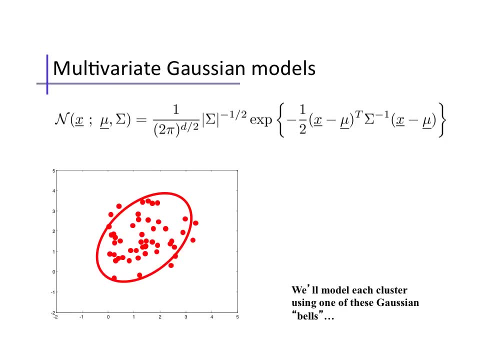 For example, in this case groups or clusters. Usually our features are multivariate, even high dimensional, So we'll typically use a multivariate Gaussian which has the same quadratic form but now involves a vector mean mu of length n, the same size as the number of features in a data point x. 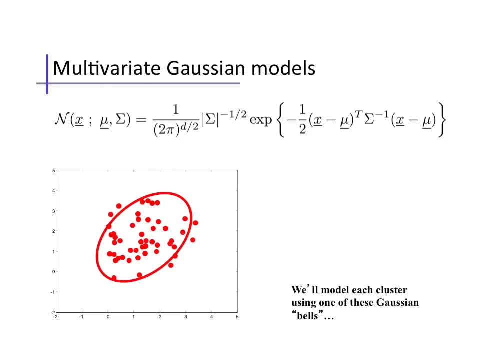 and an n by n covariance matrix sigma. Recall that if we were given data from a multivariate Gaussian, the maximum likelihood estimate for the model parameters were simply the mean of the data. so the first moment of the data and the covariance estimate. 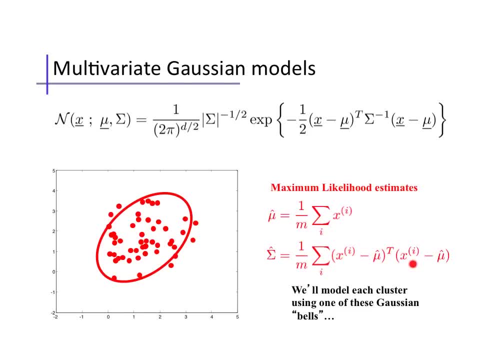 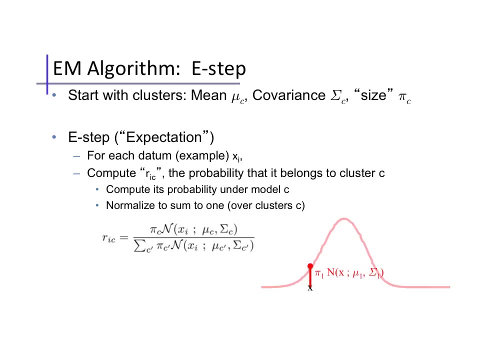 was simply the mean of the n by n matrices formed by the outer product of x minus mu with itself. So this is the centered second moment of the data. EM then proceeds iteratively in two steps: The first, the expectation, or e-step. 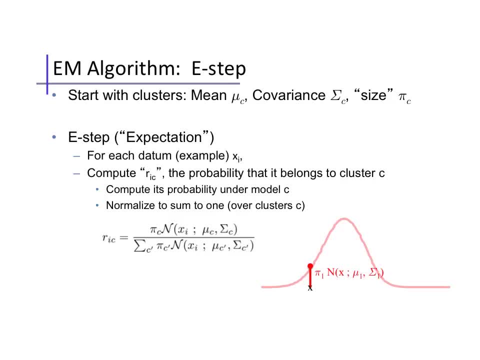 treats the Gaussian parameters mu, sigma and pi as fixed. Then for each data point i and each cluster c we compute a responsibility value r sub i c that measures the relative probability that data point x i belongs to cluster c. 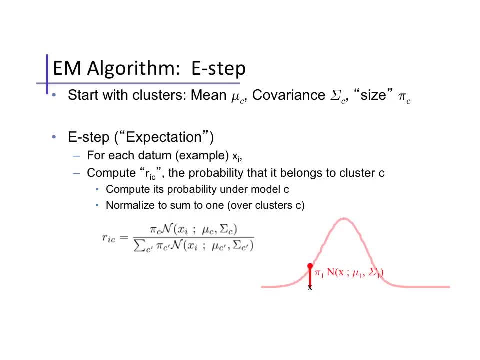 To do this we just compute the probability of x under model component c, a weighted Gaussian, and normalize by the total over all the values of c. So here we evaluate a data point, x under component one, so pi one times the Gaussian defined by mean mu one. 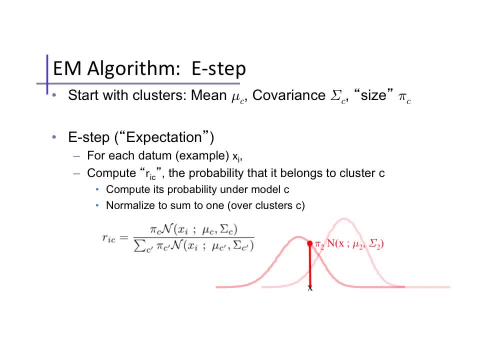 and covariance, sigma one. We then also evaluate its probability under component two. so pi two times the Gaussian defined by mu two and sigma two. If a particular component c is not a very good explanation for x, it will typically have a small r i c value. 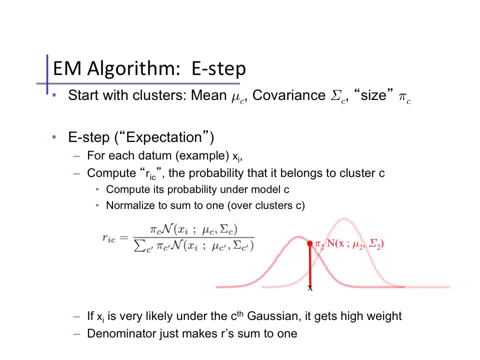 Conversely, if it's by far the best possible explanation for x, it'll have r i c approximately equal to one Here. component two is about twice as good an explanation as component one for that data point. So component two gets responsibility two thirds. 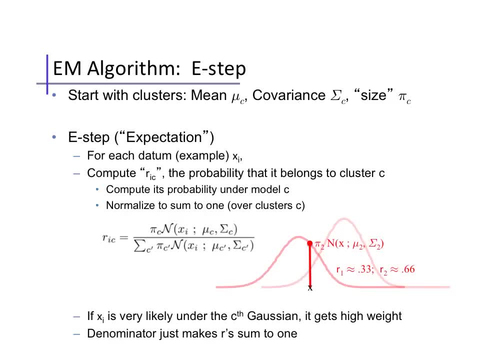 and component one gets responsibility one third. Practically speaking, r i, c is a number of data by number of clusters, so m by k matrix that sums to one over the index c. Then in the second step of EM, the maximization or m step. 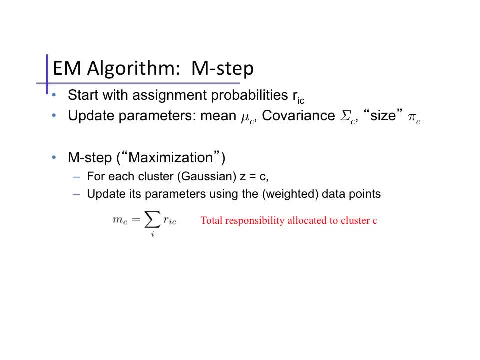 we fix these assignment responsibilities r i c and update the parameters of the clusters mu, sigma and pi. Then, for each cluster c, we update its parameters using an estimate weighted by the probabilities r i c, as if it observed some fraction r i c of data point i. 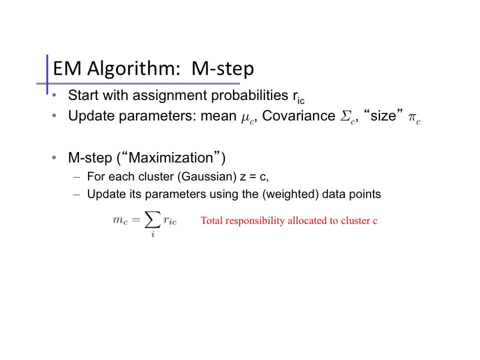 So cluster c sees some total number of data points, m c, that's the sum of these soft memberships or fractional weights assigned to cluster c. Then pi c is just this value normalized by the total number of data m. So this is the fraction of data point probabilities. 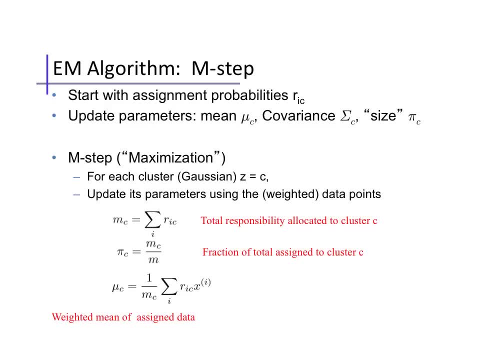 that's assigned to cluster c. The weighted mean mu c is just the weighted average of the data. So each point x- i is given weight r, i, c and we divide by the total m- c. So if a point x i was poorly explained, 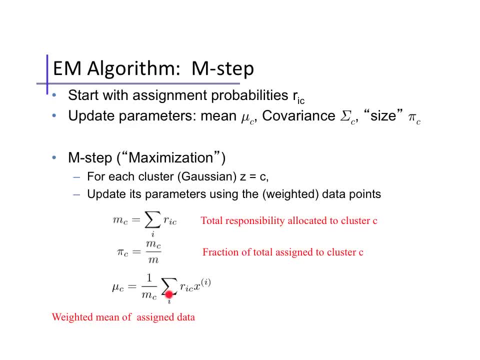 by some cluster c, its r i c will be small and that point won't influence this average very much. But on the other hand, if c was the best explanation for x, then r i c will be large and x i will influence the mean more. 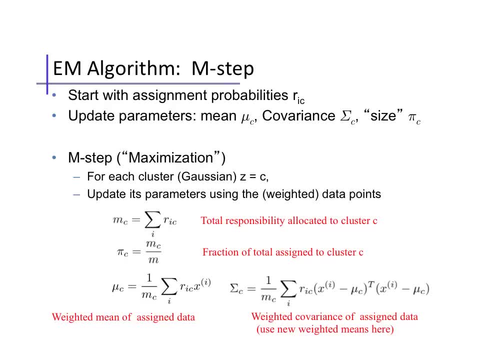 The covariance is similarly just a weighted average of the n by n matrices, formed by taking the outer product of x i minus its cluster c's mean Again, they're weighted by r i c, so that if x i is a strong member of cluster c. 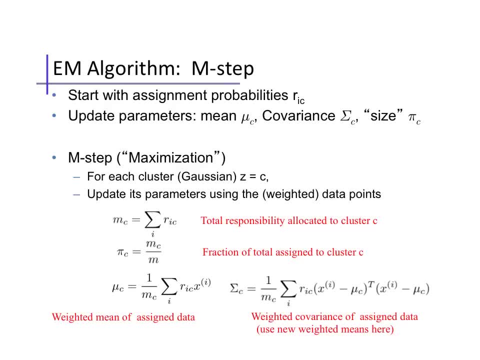 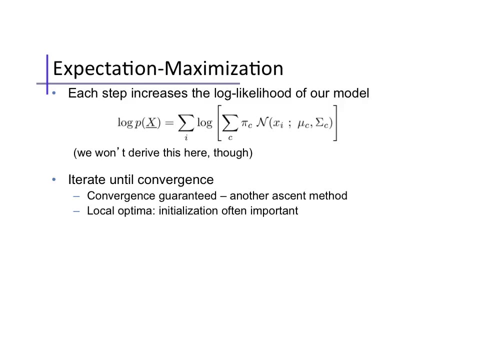 this weight will be nearly 1.. If x- i is not very well explained by cluster c, then it won't enter into this average very much. It's straightforward to prove- although I won't do it here- that these iterations strictly increase the log likelihood of the model. 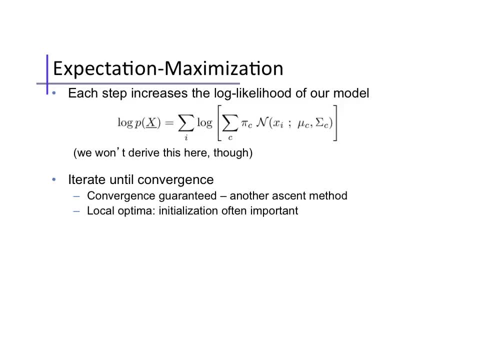 It's increasing its fit to the data. The log likelihood is just the log probability of the data points under the mixture model. So it's a sum over data points of log of the probability p of x from before, where that probability is a mixture of Gaussians. 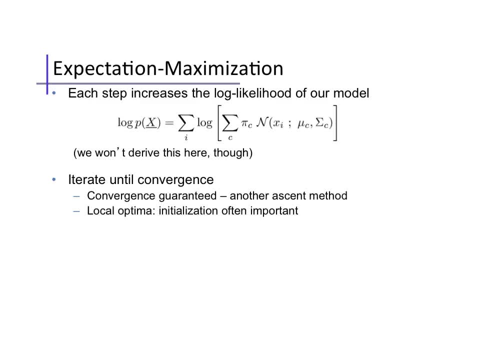 In fact em is interpretable as a form of coordinate ascent, just like our previous k-means algorithm. So thus we're again guaranteed to converge. However, convergence here won't typically be as abrupt as it was in k-means, So in practice one usually stops. 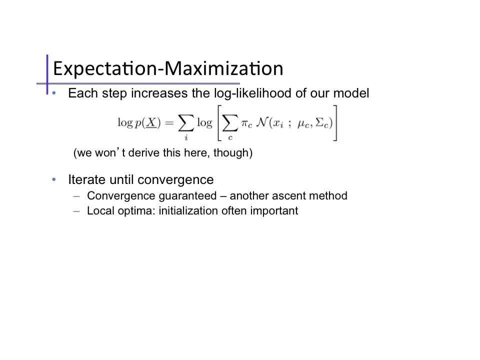 once the parameters or the log likelihood objective have stopped changing very much, Note that, like in k-means, convergence is not guaranteed to be to a global optimum, So we may have to start from several initializations and use the log likelihood to select the best. 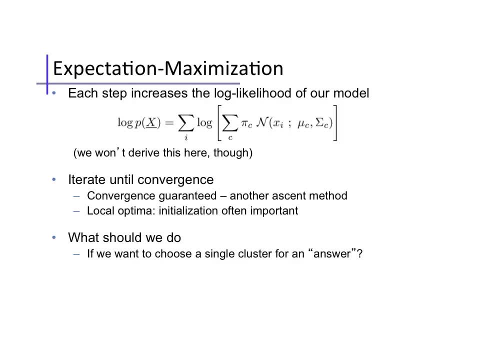 One quick point. The result of this algorithm is a description of a collection of clusters, so centers and covariances and so on, and soft membership probabilities for each data point If we want to identify our data points with a single cluster, like in k-means. 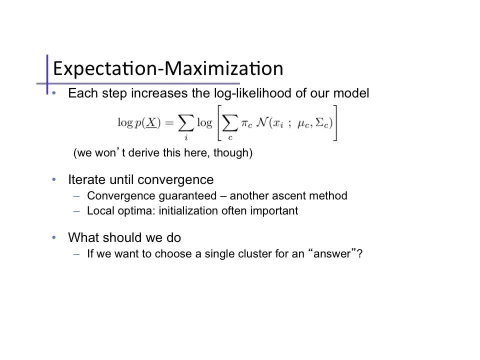 we could actually just choose the most probable cluster, so the cluster C that has largest value RIC for data point I. Just like in k-means, the view of clusters is easily applied to new out-of-sample data points as well, So these points can be given. 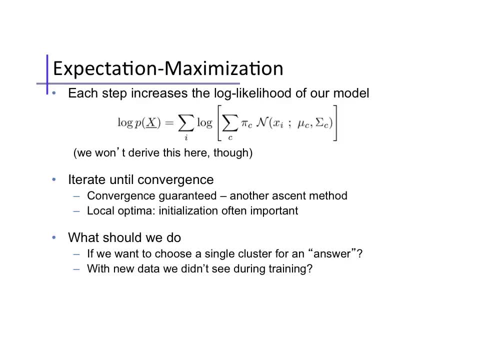 either a soft cluster membership- RIC- using an ESTEP, or a hard membership assignment- ZI- by again taking the largest value, or just RIC. Also, like k-means, selecting the number of clusters is important and can't be done using the clustered data themselves. 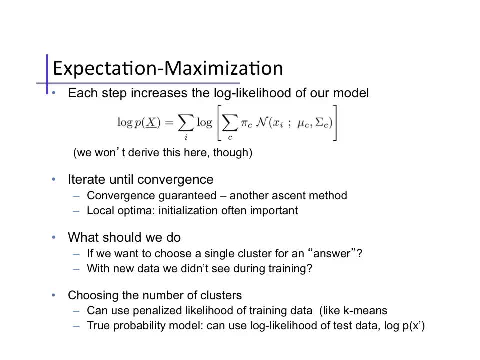 So, like k-means, one option is to use a complexity penalty in our score. An analog to the mean squared error cost in k-means is the negative log likelihood of the data in our mixture model, And we can then include a complexity penalty, like BIC. 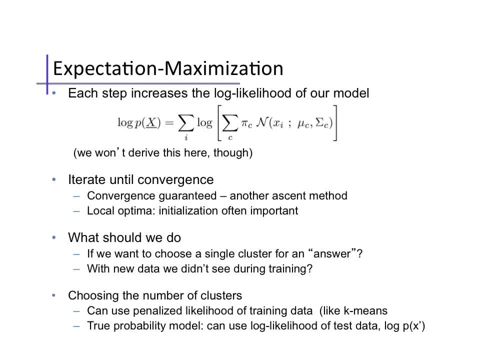 just like before. Alternatively, since the Gaussian mixture model is a true probability model, we can use the log likelihood of a validation or test set to assess the model fit as well, by evaluating the mixture probability on the new data points. Here's a demonstration of EM. 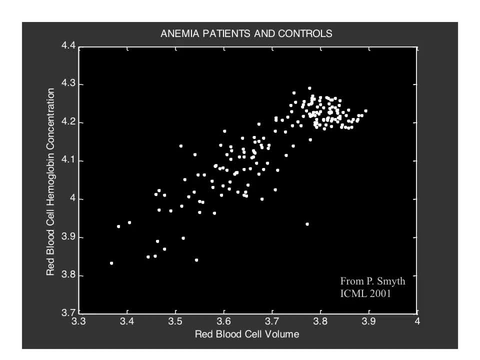 courtesy of some slides by Professor Porek-Smith here at UC Irvine run on data measuring properties of patients' red blood cells. The data include both a group of normal patients and a group of anemic patients, but the diagnosis is actually hidden from us. 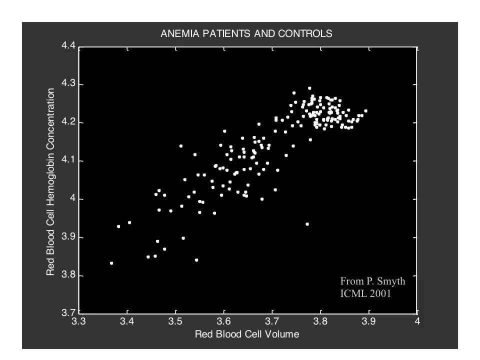 so we only see the feature measurements themselves. Probably you can see the two groups of patients already in the data Up here with high red blood cell volume and high hemoglobin are the normals and then this long dispersed group with lower volume and lower hemoglobin. 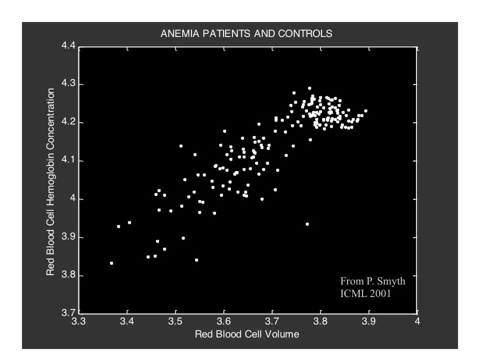 are the anemics. Let's see how EM identifies these two groups automatically. We initialize our two clusters randomly. In this case they're actually quite similar, but the means and covariance of the green cluster and the red cluster are slightly different, and that'll actually be enough. 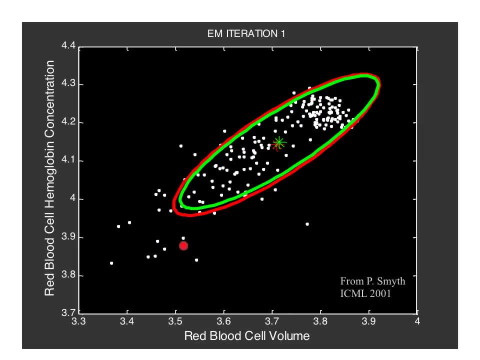 During the E-step. these points over here will be slightly more probable under the red model than the green, while these points will be about equally explained, and these points will be slightly more probable under green, Given these soft assignments or responsibilities when we update our model parameters. 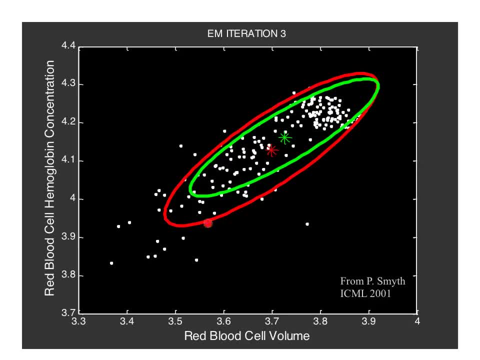 to compute the weighted mean and covariances, we'll find that the red model shifts slightly to better accommodate the data down here that were given higher probability under the red model, And similarly, green shifts to better accommodate the data that were given slightly higher probability. 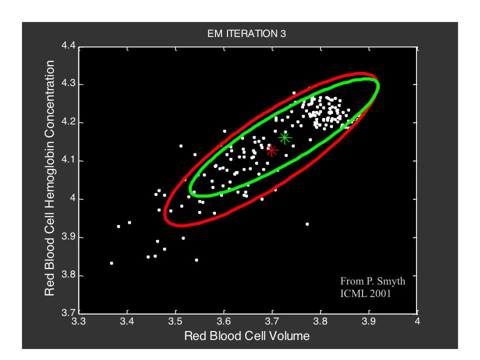 under its component. Then recomputing the probabilities in the E-step makes these data even more likely under red and these data even more likely under green. Another M-step evolves the components even further away to help explain their respective data points better. 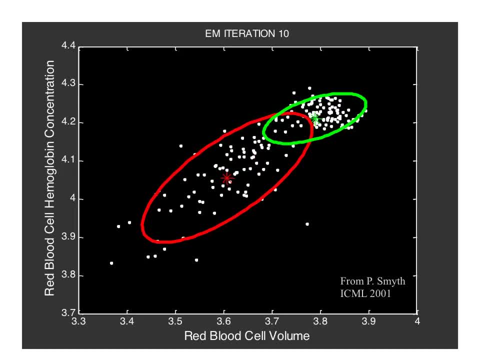 Repeating, we see that the clusters are continuing to separate. By iteration 10,, they're explaining very different groups of data and by iteration 15, red is almost entirely responsible for the dispersed data and the green cluster for the tight grouping of normals. 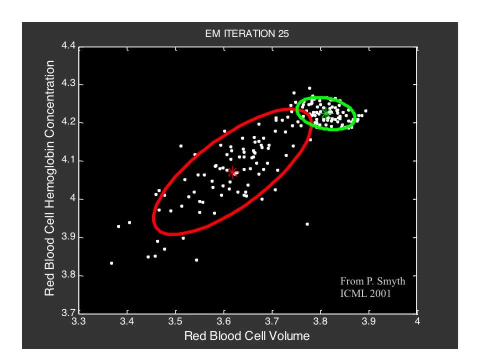 Eventually this process converges, the models cease to change very much and we can stop. Note that the model doesn't know which of these two groups is normal or anemic, Just that it can find two distinct groups or clusters in the data. 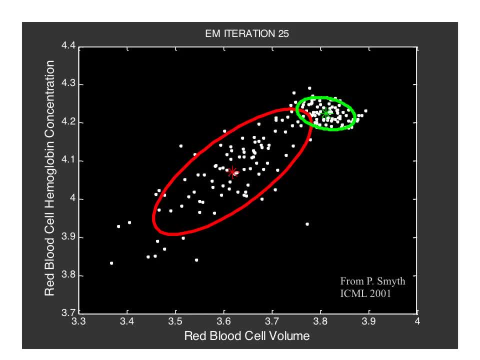 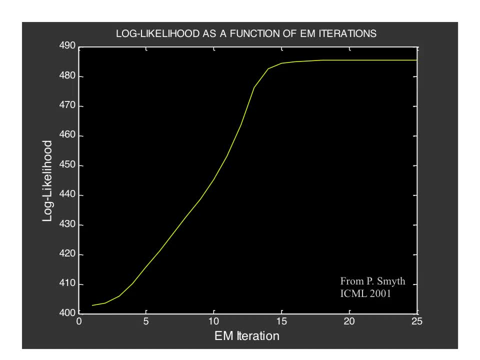 that behave differently and a description of what the data in each cluster look like. If we look at the log likelihood of the data over the course of the algorithm, we find that each iteration strictly increases the log likelihood score. So after about 15 iterations- 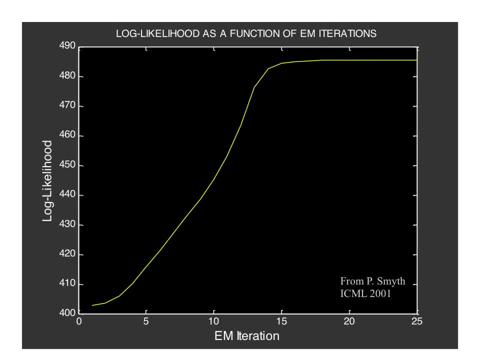 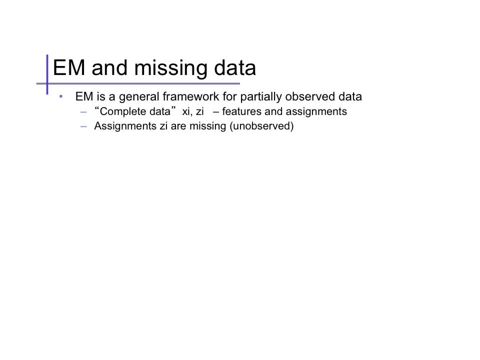 the score plateaus and doesn't increase any further, indicating again that the model has converged. The EM algorithm is actually quite general and can be used for many models or problems involving partially observed data. From this viewpoint here the complete data are the feature values. 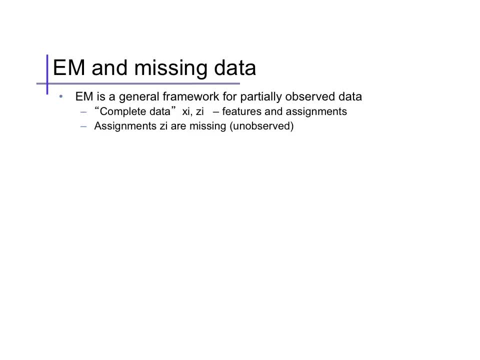 and the cluster assignments, but unfortunately for us the assignments zi are missing. Then EM corresponds to first computing the distribution over the hidden variable zi, given the current parameters of the model, and then maximizing the complete log likelihood over x and z together. 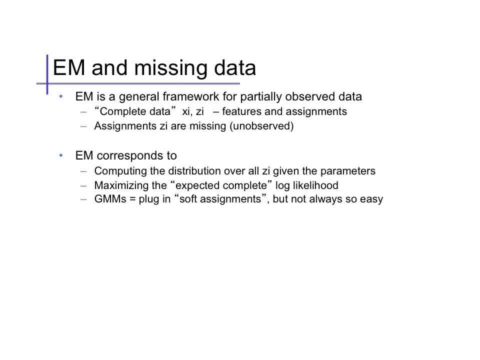 in order to determine an expectation over the distribution of zi In Gaussian mixture models. this gives us this elegant algorithm that we saw, where we compute soft assignments for each data point and then plug those soft assignments into the maximum likelihood estimates, But in more general models. 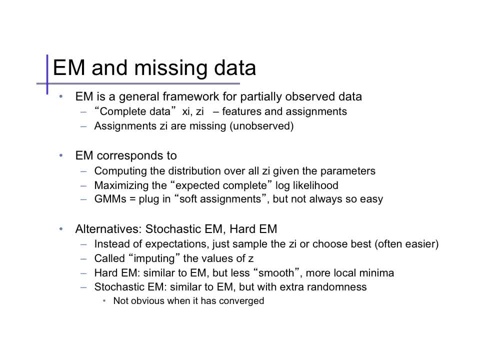 it may be procedurally a bit more complex. Two simple alternatives are often used when EM is difficult to implement. There's a stochastic version of EM or a hard version of EM. In stochastic EM, instead of taking the expectation over zi, we just sample its value and then fix it. 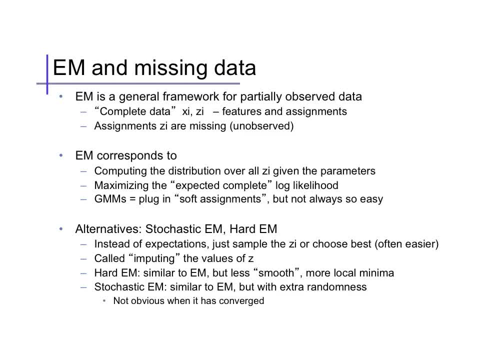 In hard EM we select the most probable value and fix it. Often it's easier to work with a fixed value of zi than maximizing the expectation. This process of plugging a value into zi is often called imputing the value of zi. 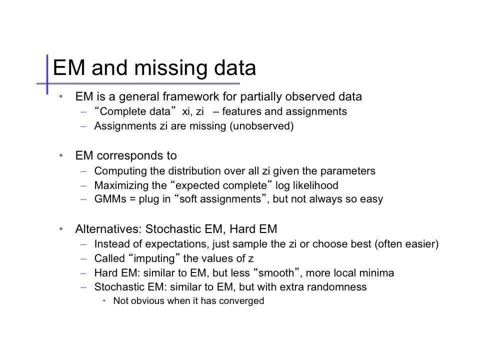 Both variants, stochastic and hard EM, are quite similar to regular EM. Hard EM, as you might imagine, is a little less smooth in its optimization, since the best value of zi might change discontinuously, and it's often prone to more local optima. 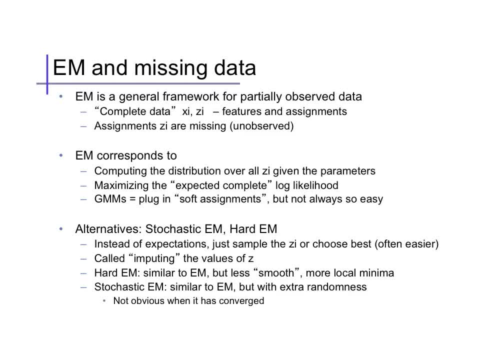 since once we have a hard assignment, we'll move the parameters to explain it, which then reinforces that hard assignment. Hard EM is very closely related to k-means. with this best assignment update, Stochastic EM is less prone to local optima but has more randomness built in. 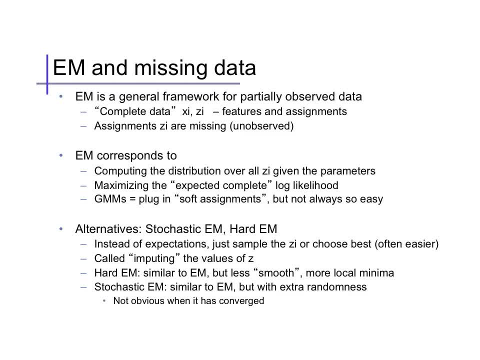 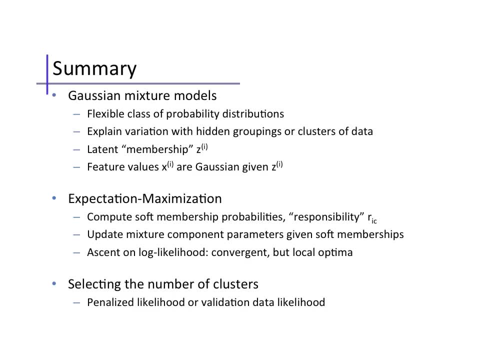 making it harder to gauge convergence. In summary, Gaussian mixture models are a useful and flexible class of probability distributions. Here we're using them for clustering. They explain the distribution of the data x using a latent variable framework. So we posit that there's some hidden grouping. 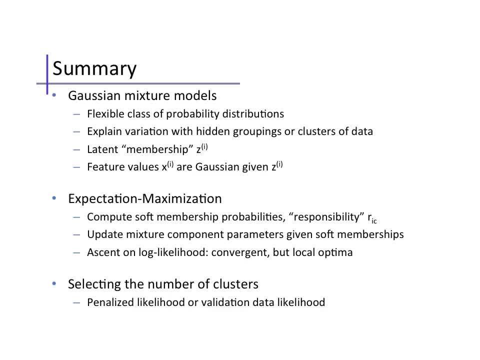 or clustering. that explains a lot of the variation in the data. Our model then contains a latent membership or assignment variable, zi, and then the actual feature values xi are Gaussian. given that cluster assignment zi, We can learn the parameters of a Gaussian mixture model. 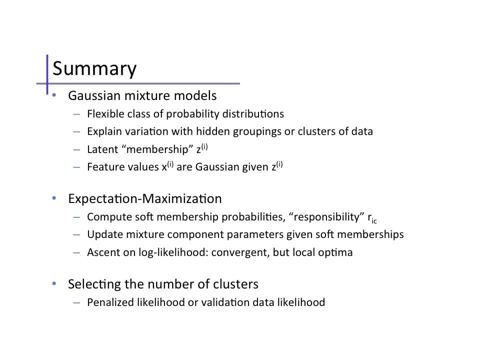 using expectation maximization or EM. EM applied to Gaussian mixture models has a simple and elegant form. We just iterate between computing soft membership or assignment probabilities, which we call the responsibilities R, sub i, c, and updating the parameters of the mixture model components. 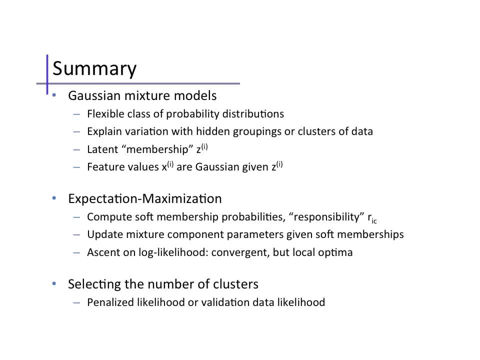 so the cluster centers, covariances and so on. using these soft memberships, This procedure is guaranteed to strictly increase the log likelihood, decrease the negative log likelihood of the model on training data, which ensures that it's convergent but it's non-convex, so it may have local optima. 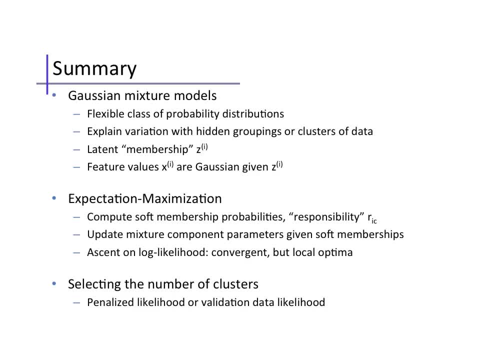 which makes initialization potentially very important. We also discussed how we can set the number of clusters using either a complexity penalty like BIC, just like we did in k-means, or, since the Gaussian mixture model is a true probability model, over x.